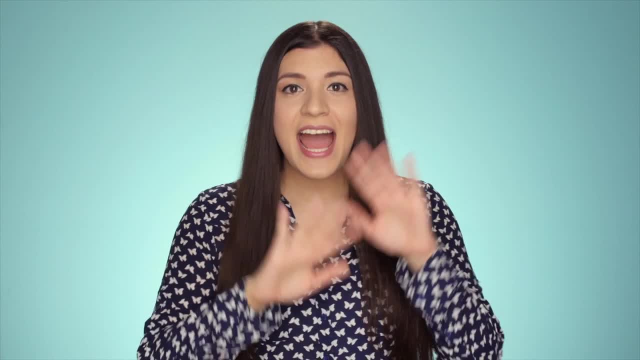 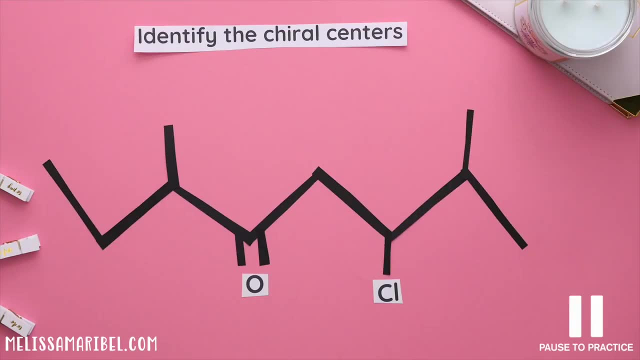 it chiral? Okay, to make sure you fully understand everything we just covered, try these two questions and we'll go over the answers in just a little bit. Identify the chiral centers. To finally answer to question one, let's check each carbon and see if there are four. 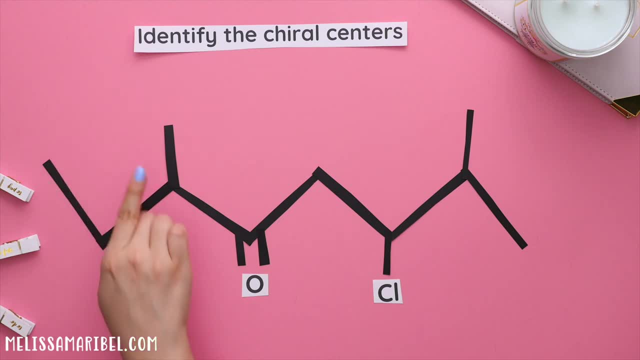 different groups. Nope, not enough groups. Not enough groups for the next carbon. This carbon has one, two, three, four different groups. so, yes, this is a chiral center. Next, remember, a double or triple bond will never be a chiral center If there are four groups. then it is a chiral center. 是不是 that's a chiral center? In fact, it's not even a chiral center. Well, I'm not sure I can say this, but I think the answer is no. So let's do a question one. 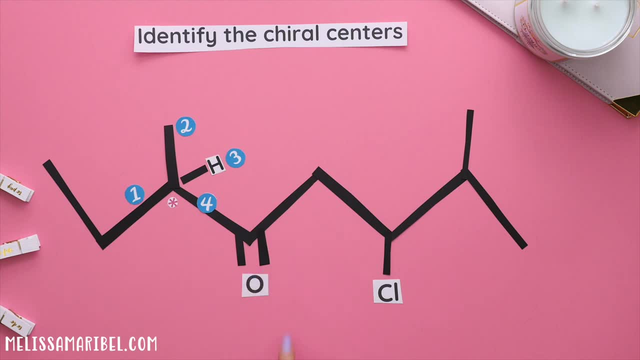 To end the question, let's check each carbon and see if there are 4 different groups, be a chiral center. so this one is not a chiral center. This next carbon doesn't have enough groups. The next carbon has one, two, three and four different groups. 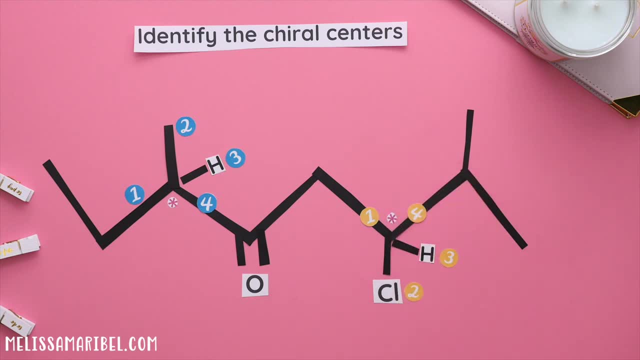 so, yes, this is another chiral center And this N carbon is a common mistake. It has enough groups, but there are two of the same groups, our methyl groups, But we need all four groups to be different. so this is not a chiral center. There are 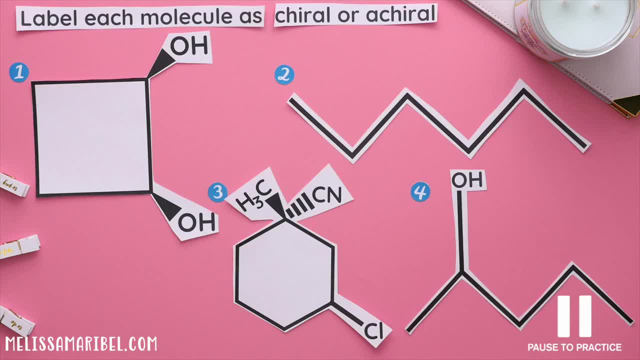 only two chiral centers in this molecule. For question two, label each molecule as chiral or achiral. To find the answer to question two, remember we are looking for lines of symmetry. If there is a line of symmetry within the molecule, then it's. 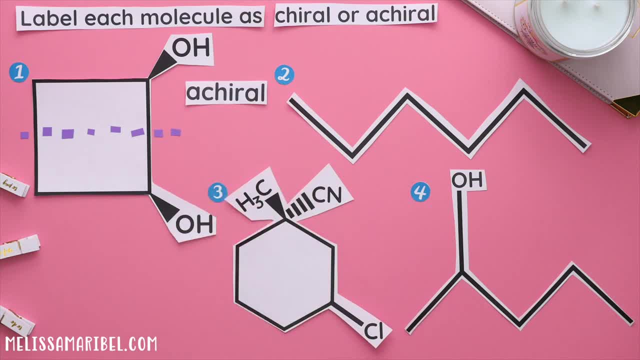 achiral. like this first one is, Here is another hidden line of symmetry. We can count the number of carbons on either side and see that we can cut this molecule in half. If there is a line of symmetry within the molecule, then it's. 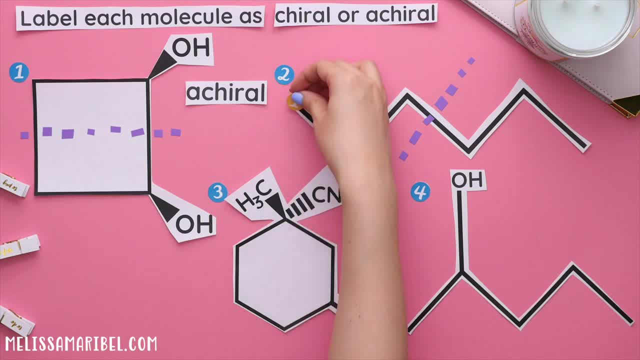 achiral like this first one is. Here is another hidden line of symmetry: We can count the number of carbons on either side and see that we can cut this molecule in half. and it would be the same, since there are one, two, three carbons on the left and one, two, three carbons on the right, making this molecule achiral. Now for the remaining. 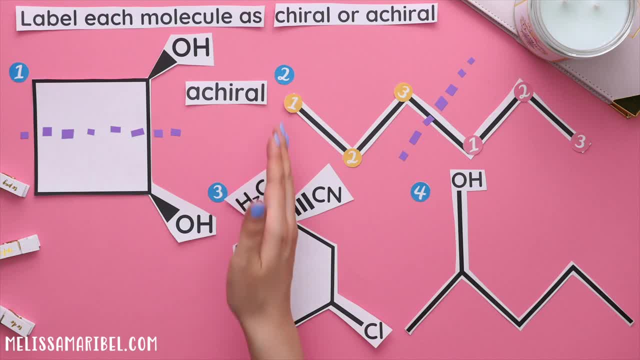 molecules there is no line of symmetry. No matter how we try to cut them down the middle, they are never the same. so these both are chiral. You can find other helpful videos right here and, if you would like additional homework help,